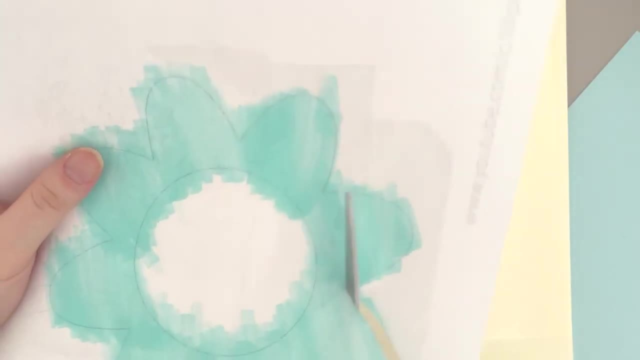 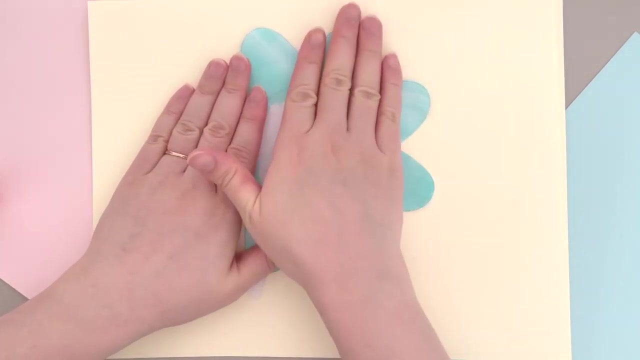 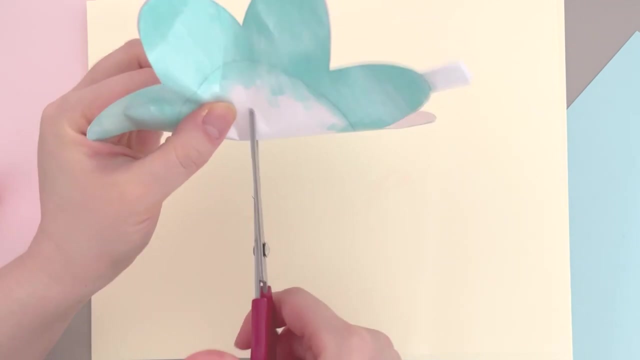 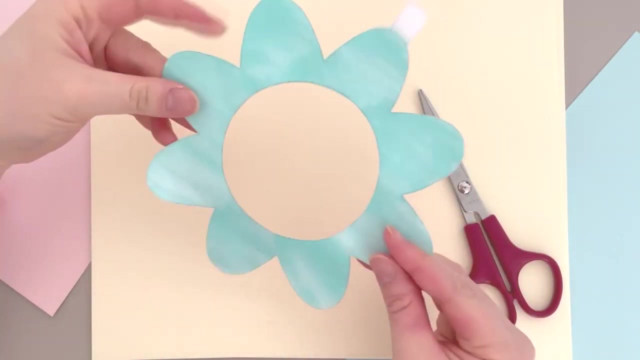 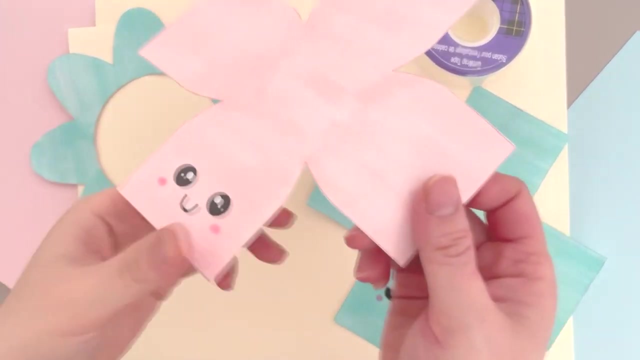 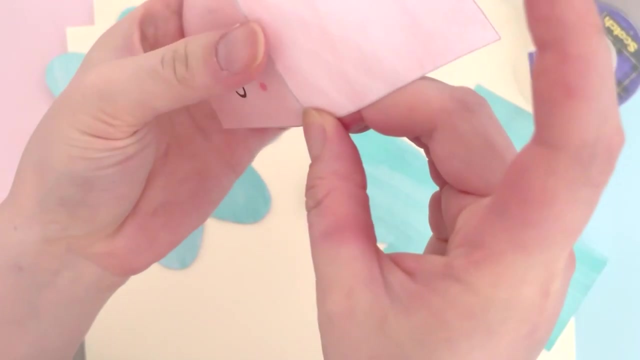 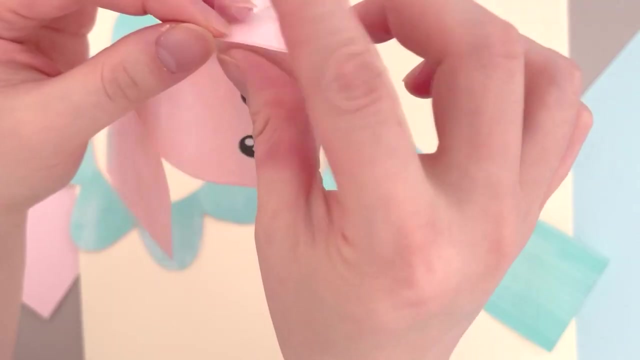 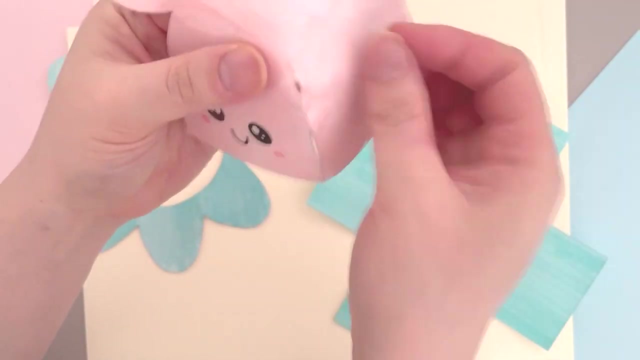 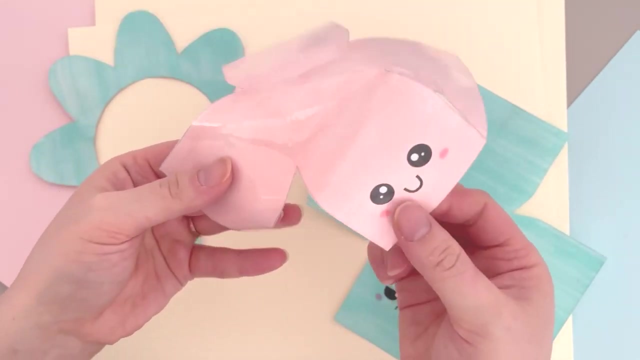 degrees to skinny. Cut out the template along the outline 탄 strength. Attach two octopus legs. cut out front and back by gluing. Connect the template along the side lines with transparent tape. Use a plastic replacement tape to seal the inside of the octopus leg. 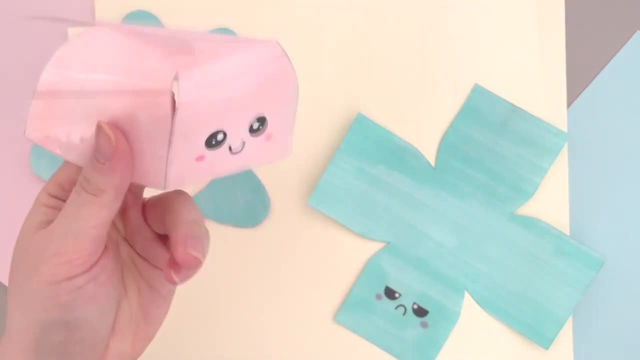 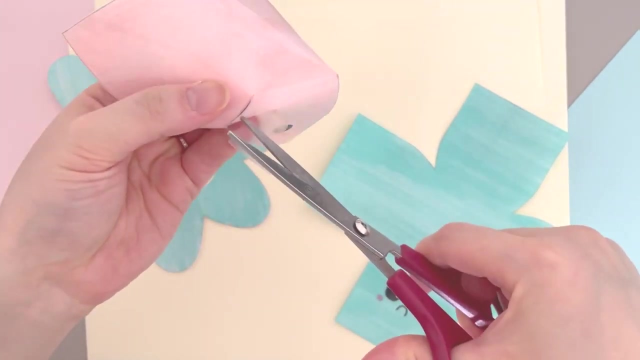 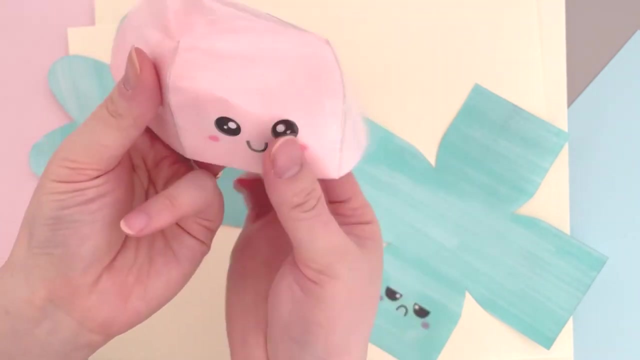 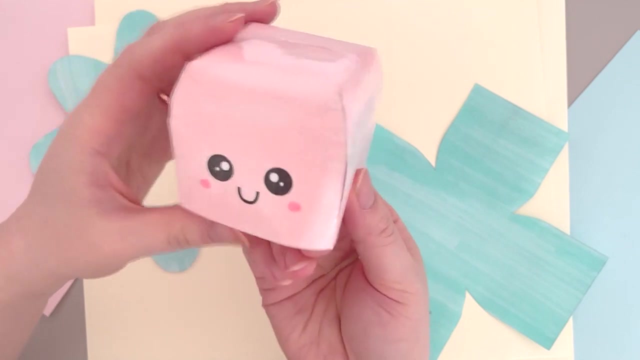 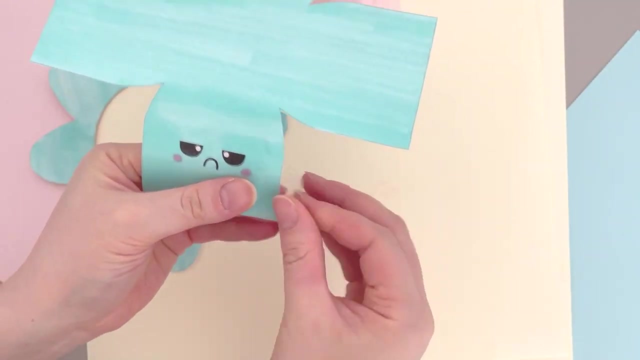 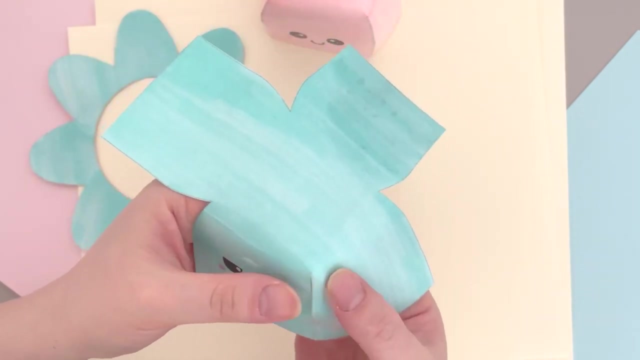 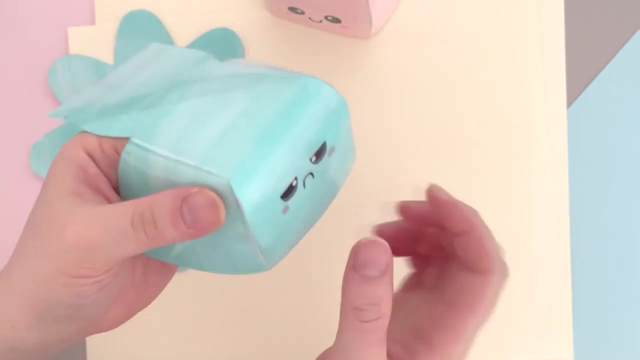 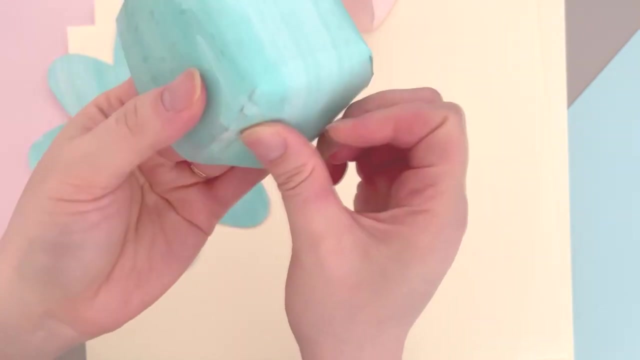 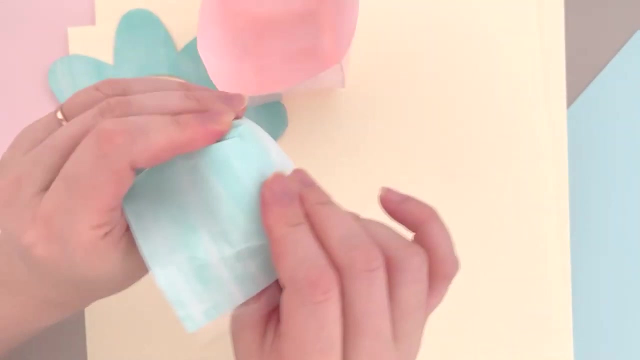 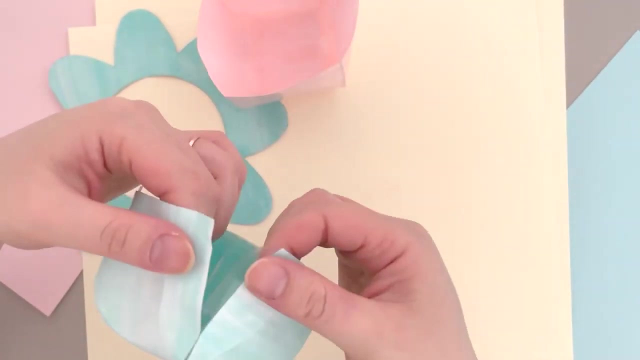 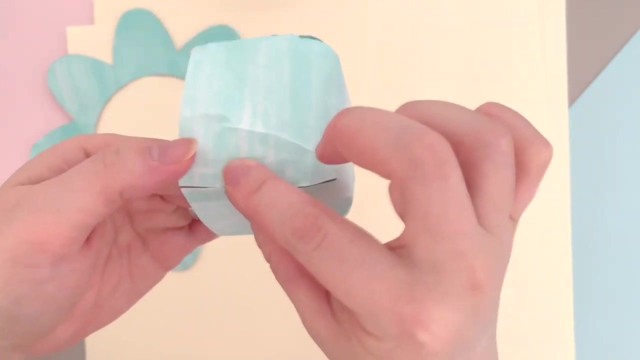 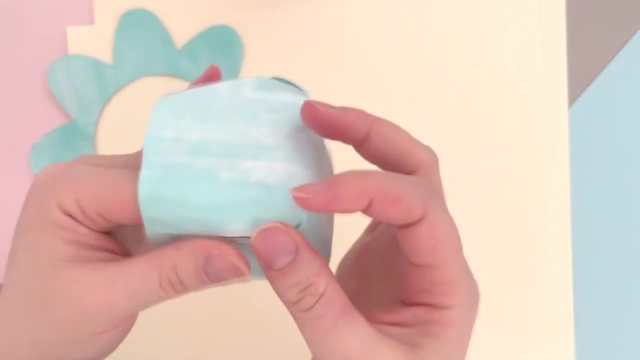 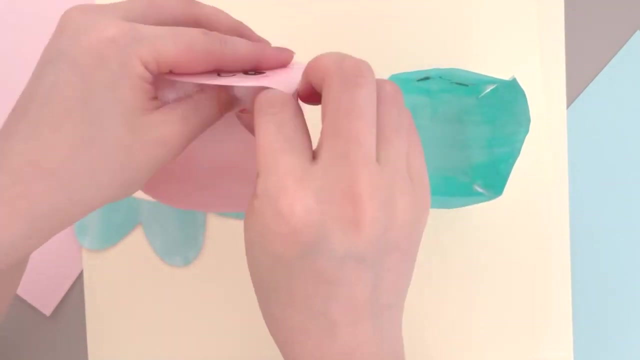 Use a black plastic wrap to seal the inside of the octopus leg. Be careful not to cut too deep. Be careful not to cut too deep. Thank you, Flip one of the heads. Insert cotton in between two heads. If you don't have cotton, tissue paper would work as well.